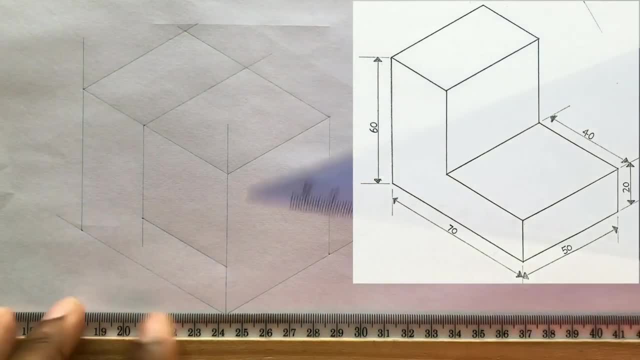 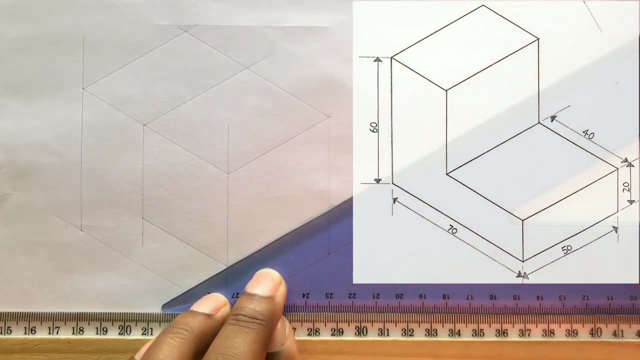 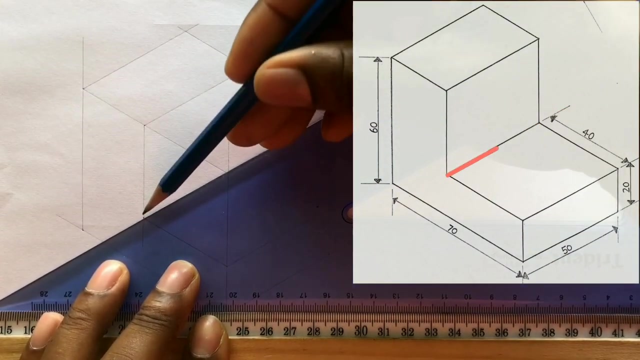 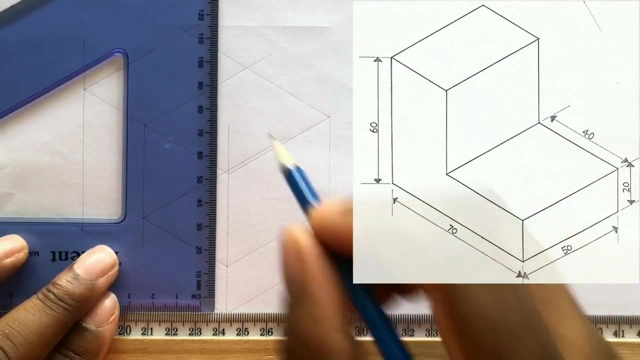 Now, from this latest intersection, you will also draw a line using your t-square and your set-square. Now, use your set-square along with your t-square and draw this line, a line from this intersection Now. you now need to draw a line from this. 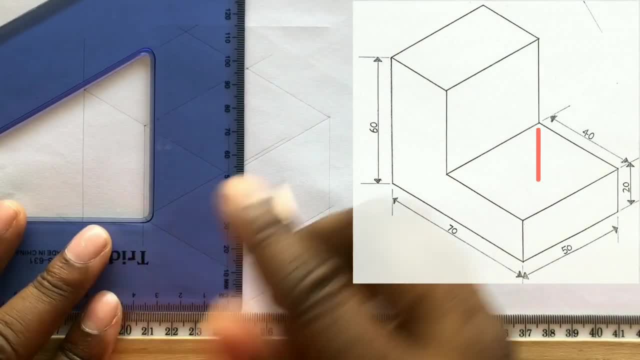 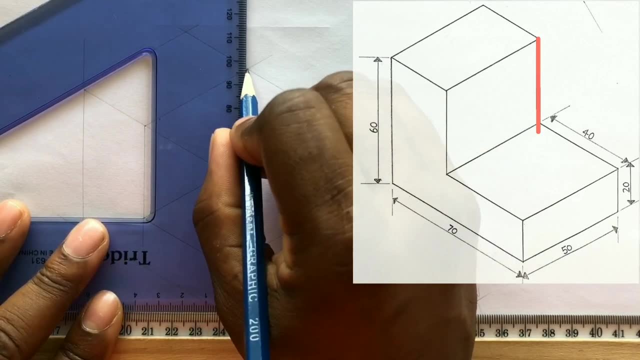 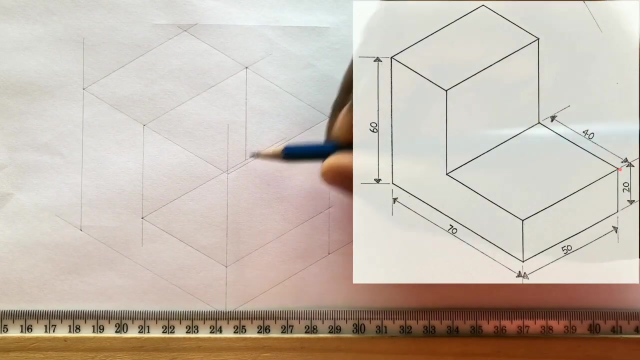 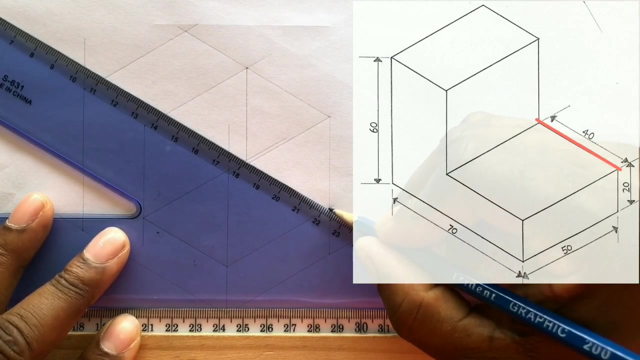 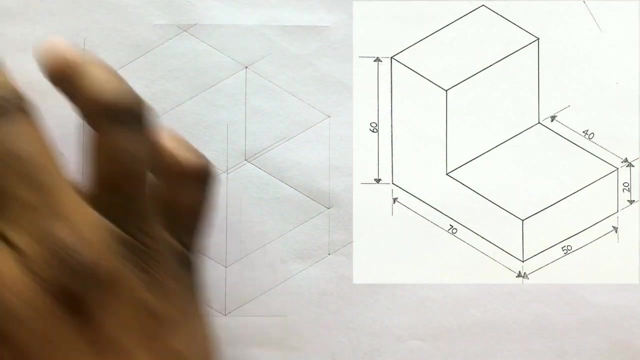 intersection vertically. This will be done using your set square and your t-square. Now your final step is to draw a line from this point to this point. Once you are accurate with all previous steps, then this line will perfectly intersect at both points. Excellent, Go ahead and outline your required. 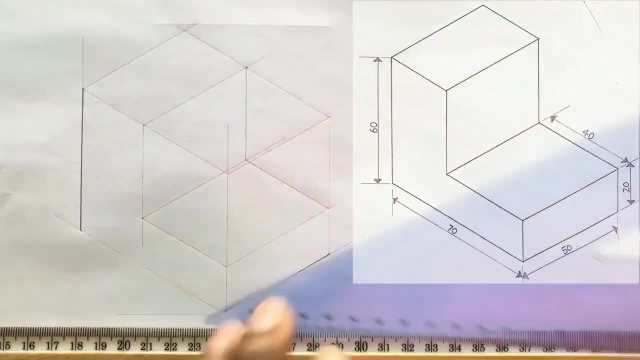 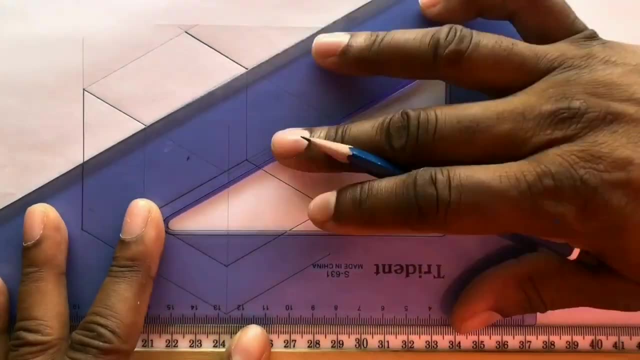 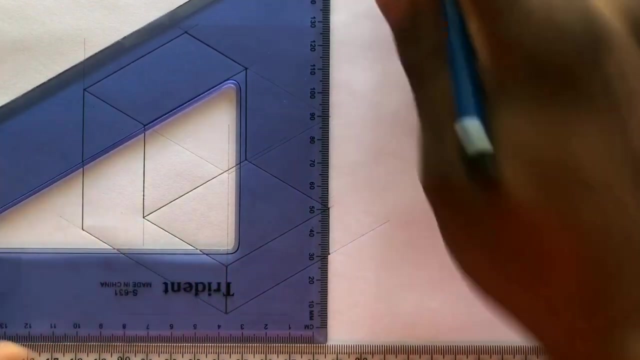 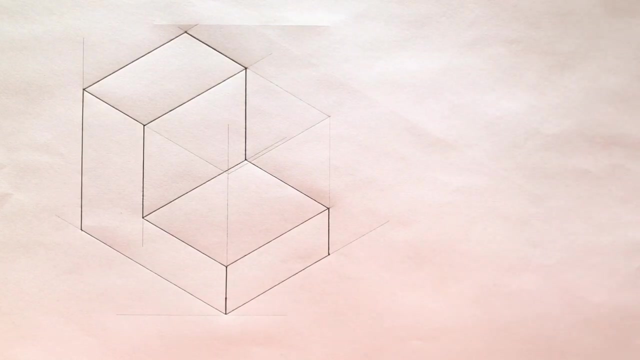 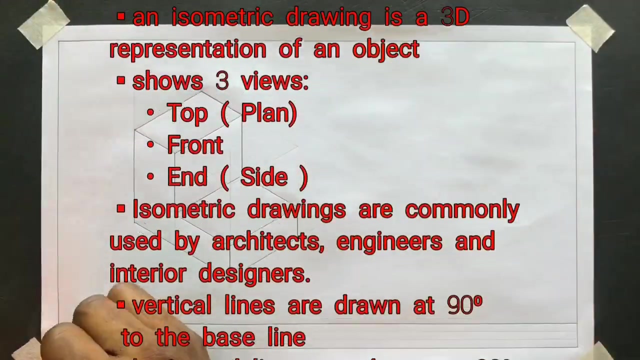 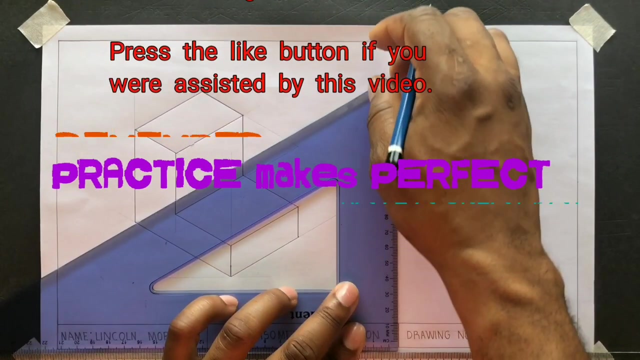 isometric projection. It was surely not difficult at all. Go ahead, border your paper and complete your title block. 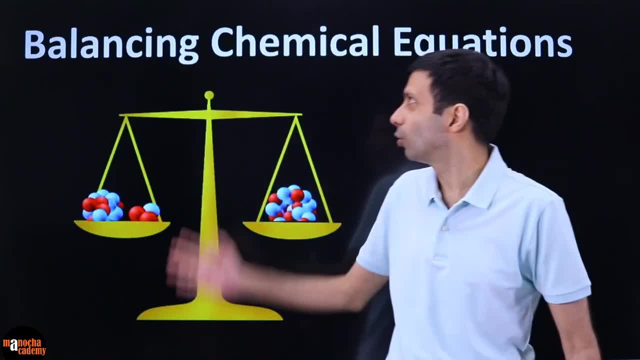 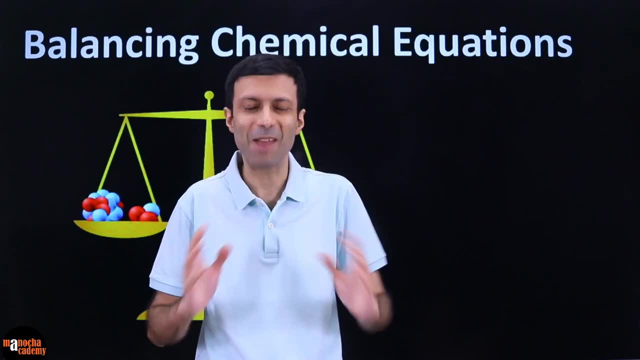 Hi everyone, welcome to this chemistry class where we are going to learn how to balance chemical equations. Balancing equations is a very, very important thing which we must know and master, and I'm going to make it really easy for you. I'm going to show you the different techniques on how to balance, and which. 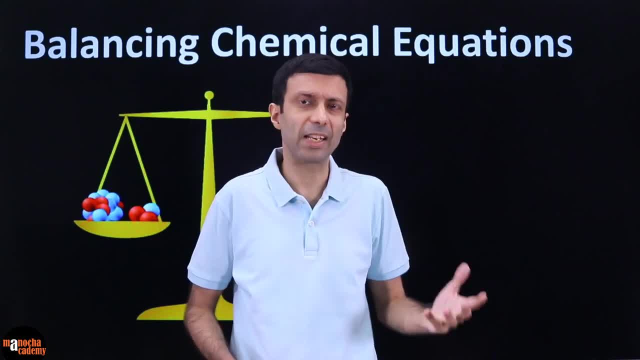 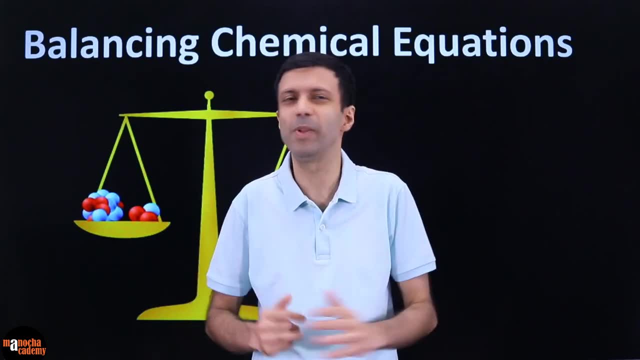 one I would recommend, because always this confusion is there. you know, which technique should I use, which one is the fastest if I get stuck, which one should I switch to? I'll answer all of that and I hope you'll be able to balance equations very easily after this class. so keep your pen and paper ready, because